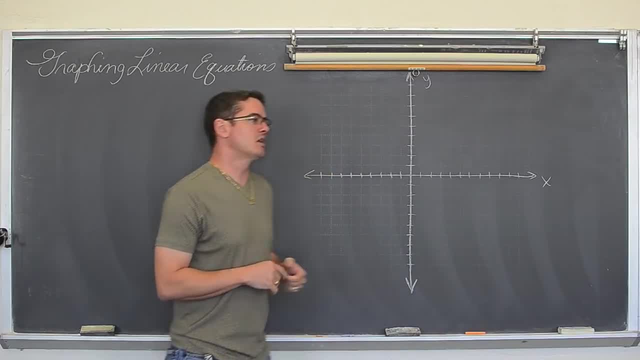 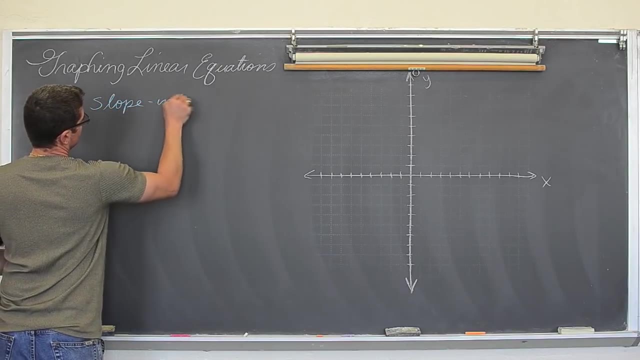 so simple if you are in Algebra 1 and you are watching this video. So let's take a look at graphing equations of lines in the most common form of equations that we use, which is called slope intercept form. Alright, so we have slope intercept form, Now slope intercept. 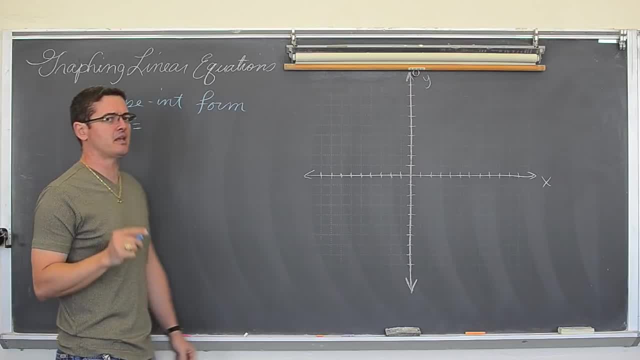 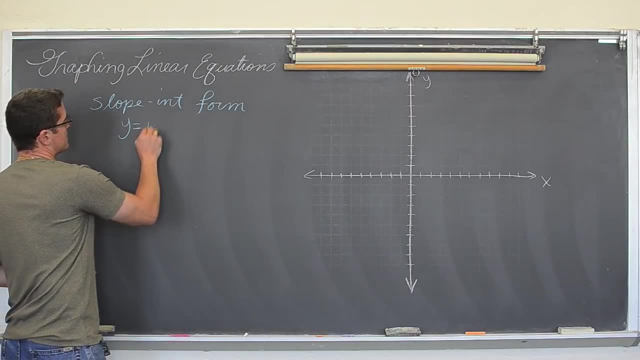 form is in the form of, that is, when you have y by itself. That is the biggie. Almost every time you have an equation where y is alone, you are probably going to be in slope intercept form. That is: y equals mx plus b. 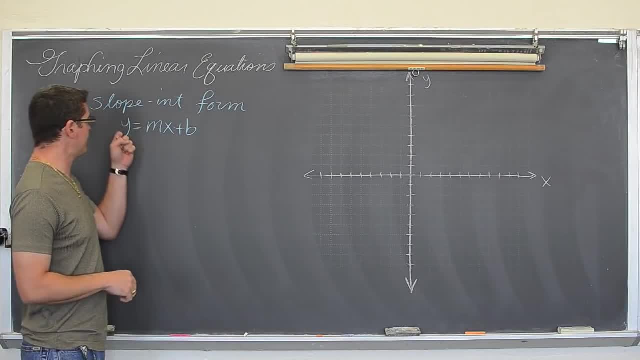 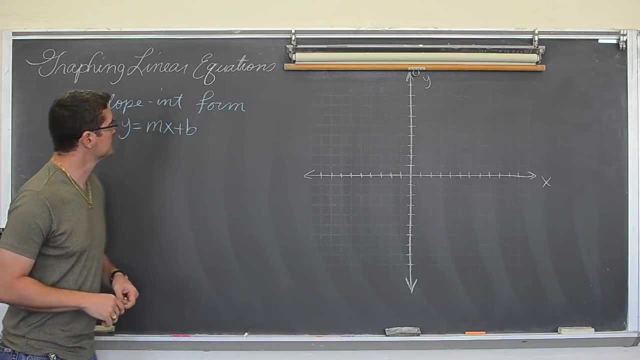 Now note that there are no parentheses in here. So if you have an equation where y is by itself but there is parentheses in there, you will need to get rid of those before you try and graph it. We really like graphing in this form because when y is alone, you 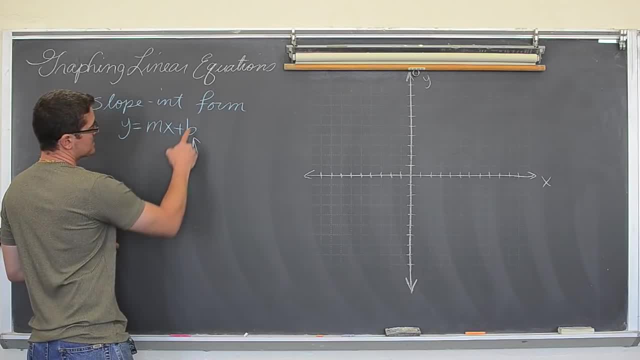 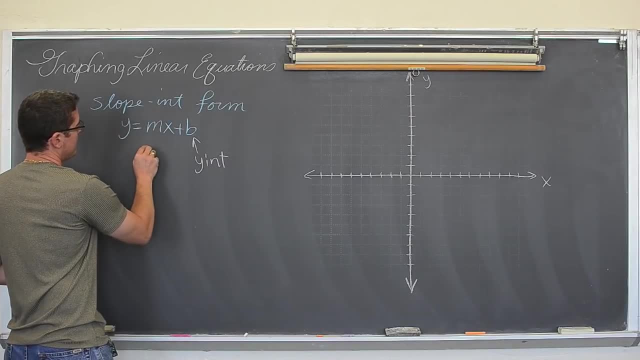 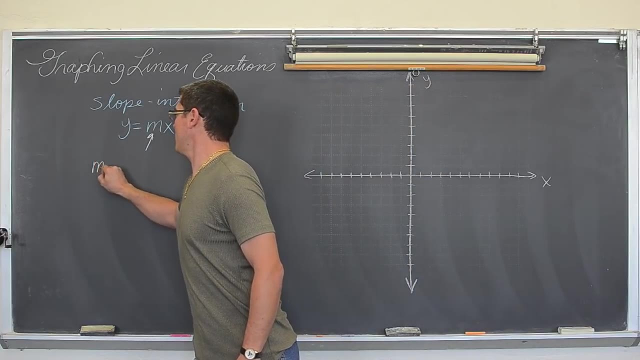 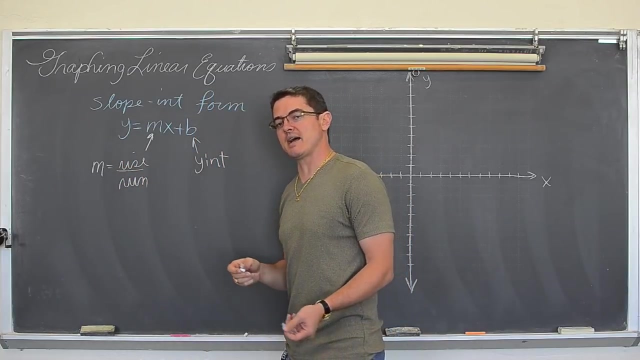 are looking at b, the constant, the number that does not have or is not with the variable. This is your y intercept. And m, or the number that is immediately in front of the x, is your slope. So slope is rise over run and there is also an equation attached to slope. 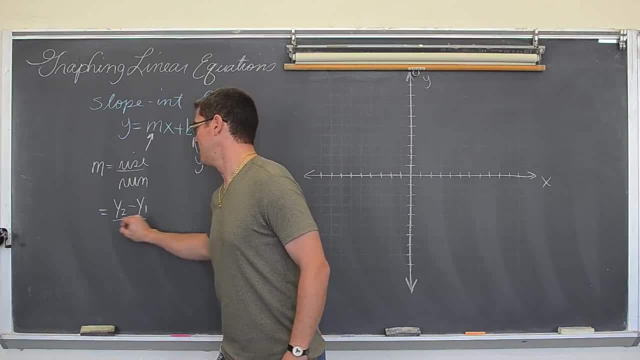 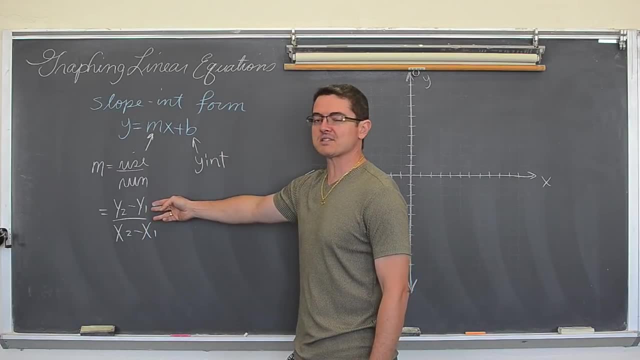 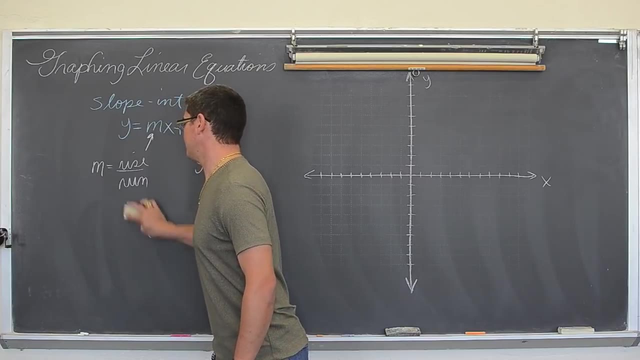 which we are not going to be using today, but it is y2 minus y1 over x2 minus x1.. Ok, so slope is rise over run. Your y axis is your up and down movement. So when you subtract you will find your rise and your run value. I like to teach graphing. 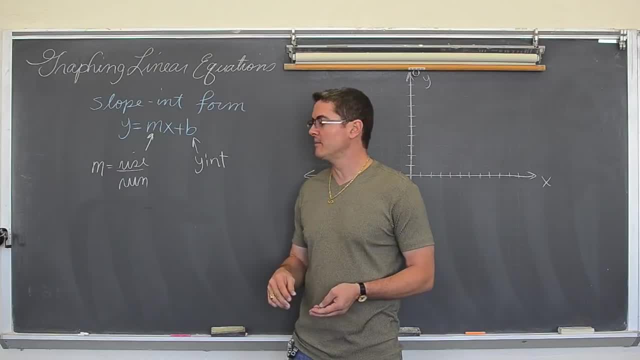 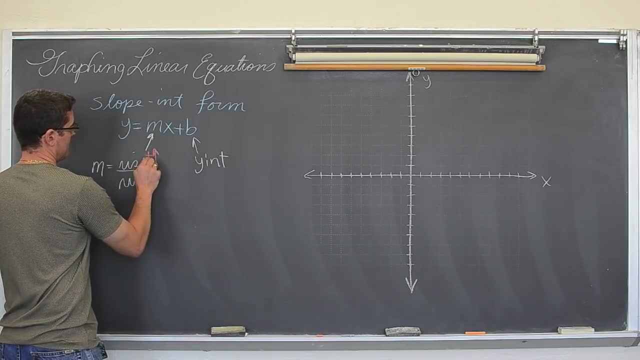 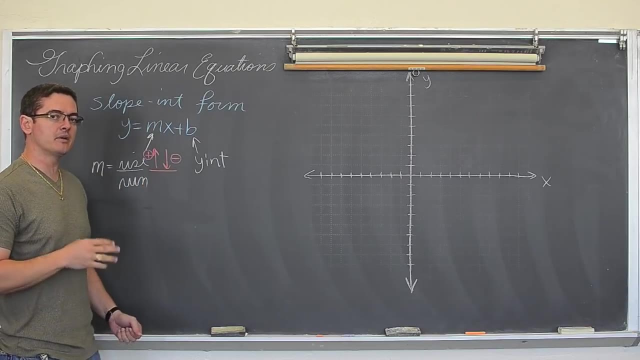 And teach slope as if you are reading a book. So if your slope is positive, you are going to be going up for a positive slope and down for a negative slope. Now this is not an absolute requirement but again, I think it just makes it a little bit easier If you think of slope. 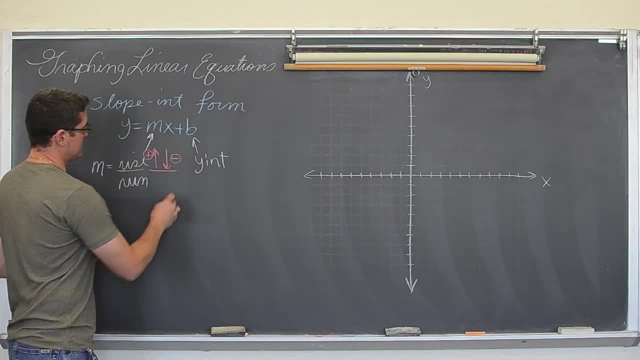 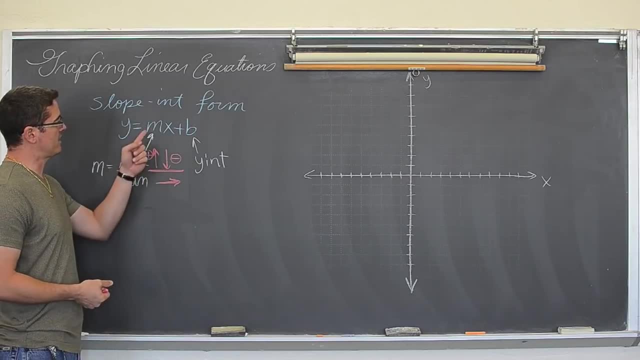 as reading left to right, then it will not leave any doubt that your run is always to the right. We are going to be graphing some lines and when this slope is negative, I am going to go down. When this slope is positive, I am going to go up, But the bottom number I am. 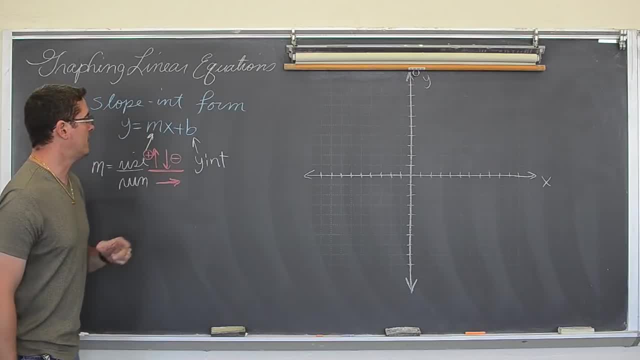 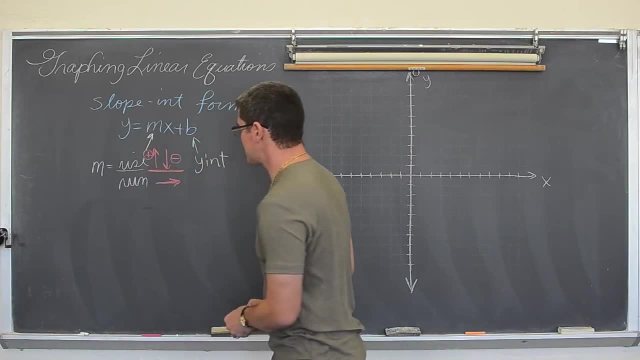 going to hold is a consistent direction to the right. Again, it is not absolutely mandatory, it is just that I found it to be easier for when I am graphing. Ok, so let's just do a couple of examples here that are already set up in terms of y or y in terms of x. Let's 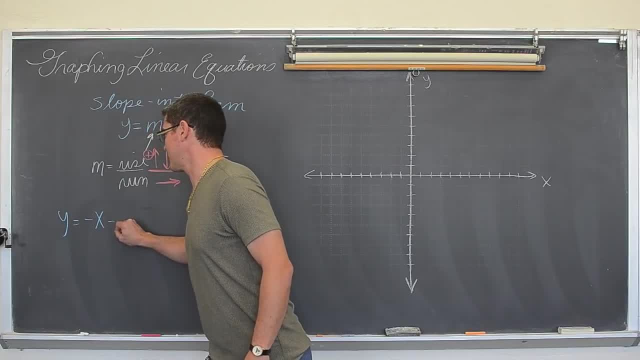 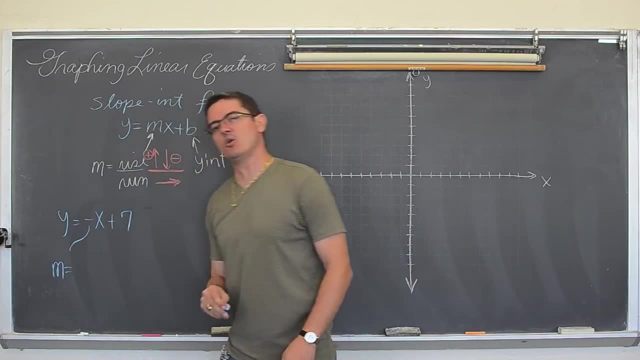 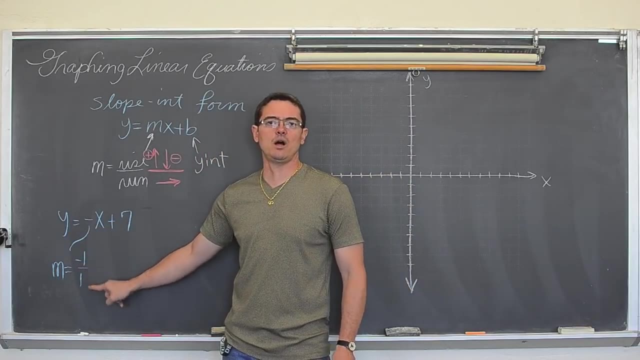 do a blue one here first. y equals negative x plus let's say negative x, So this is negative x sub 7.. Ok, well, this has a slope of negative one over one. Now, I don't see a fraction there, so I am going to write it as one over one, because a lot of students 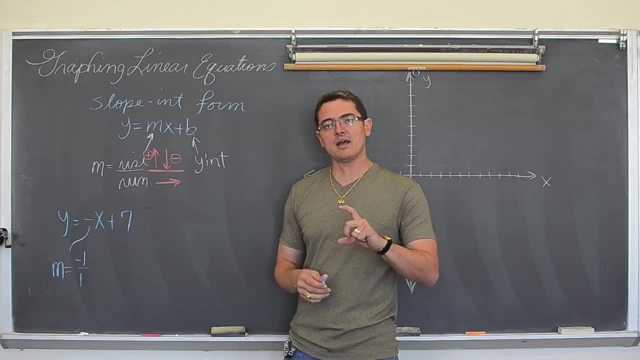 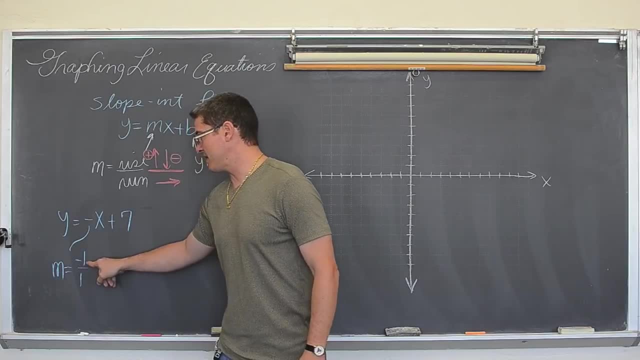 are nervous with fractions Because with slope you do need a rise and a run value, So you need to make that look like a fraction, even if it is not in your problem, And because the slope is negative and I also know you might not know where the one came in the first. 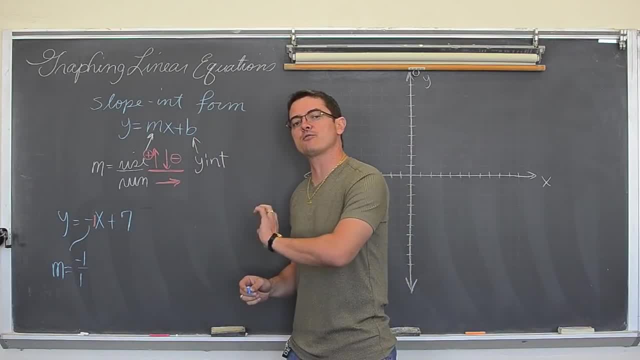 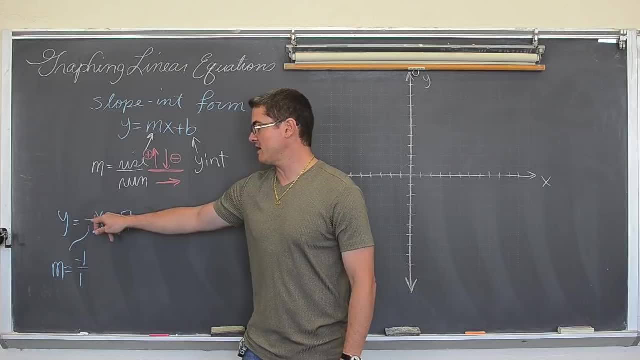 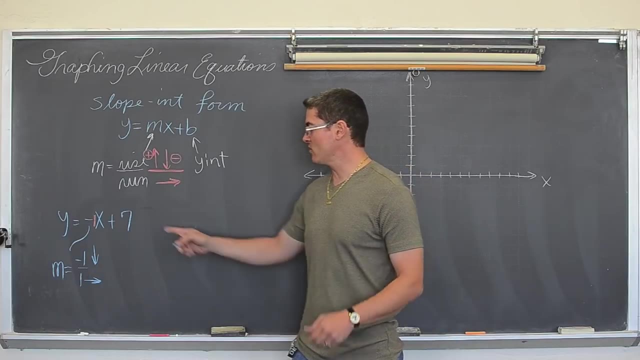 place came from. If there is nothing written in front of an x, or any variable for that matter, you always want to assume and know that there is a 1 there. So this negative x or negative 1x is going to have a slope where you go down one and over one, Always to the right, And 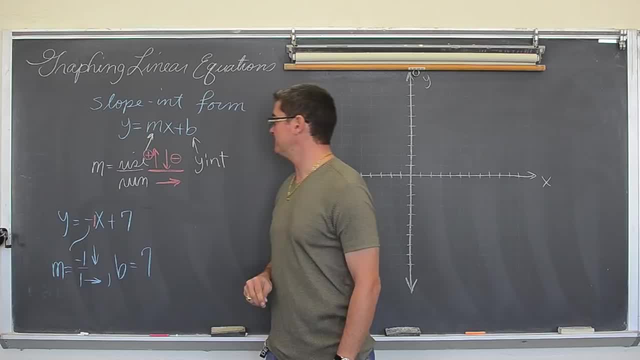 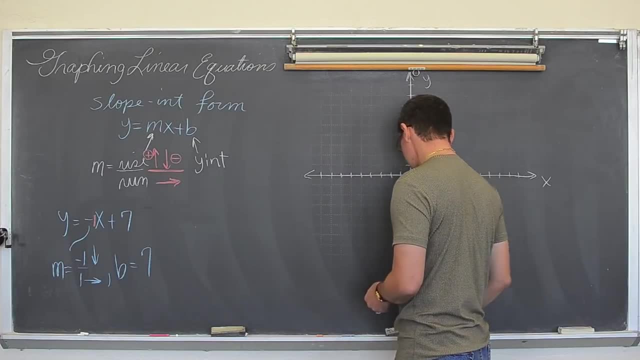 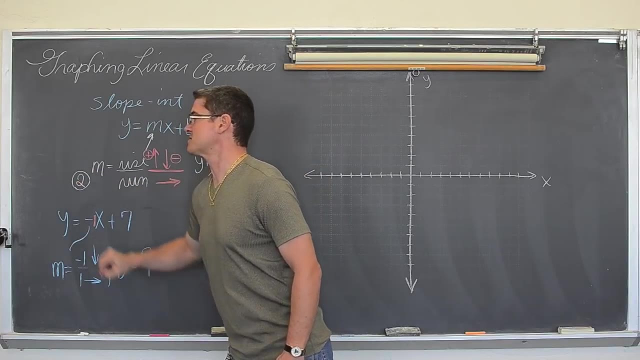 your y intercept is b, which is 7.. Now something else to think of in slope intercept form. when you are graphing- and we are doing these without the help of t tables- is you always want to do the y intercept first and the slope second. So this line is going to cross the y axis. 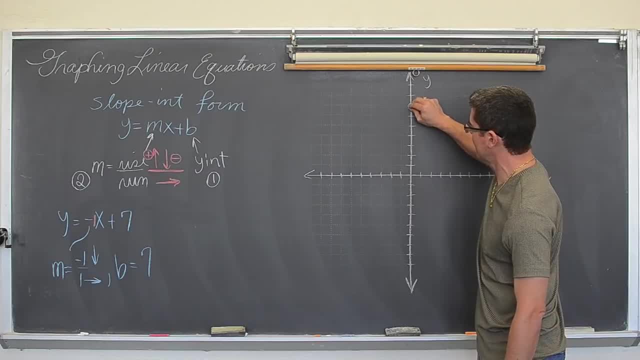 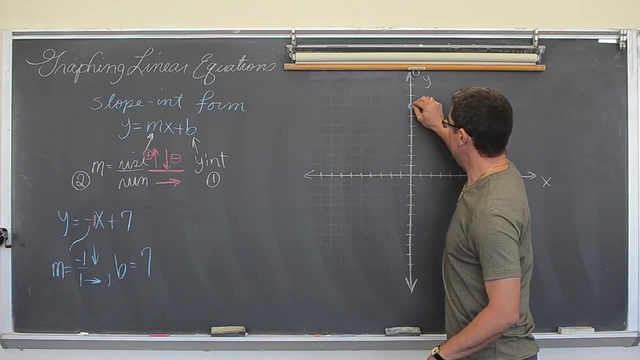 at 7.. So 1,, 2,, 3,, 4,, 5,, 6,, 7.. And from there, because there is a negative in front of the x, we are going to go down one and over one. So down one and over one, Down one and over. 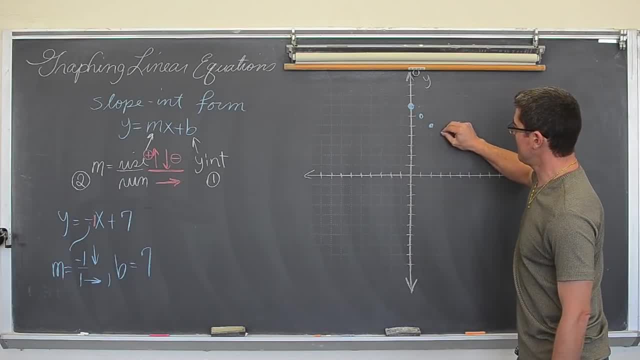 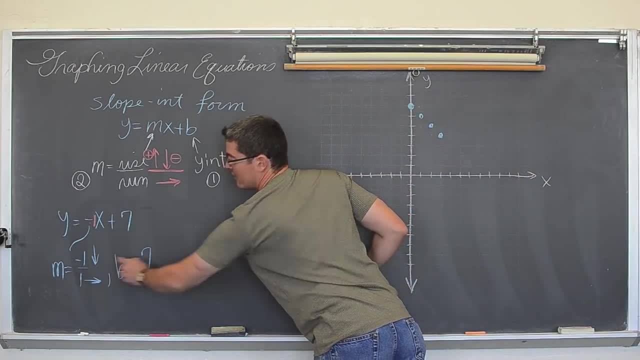 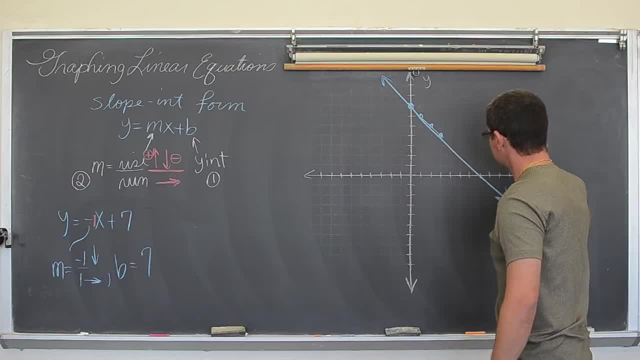 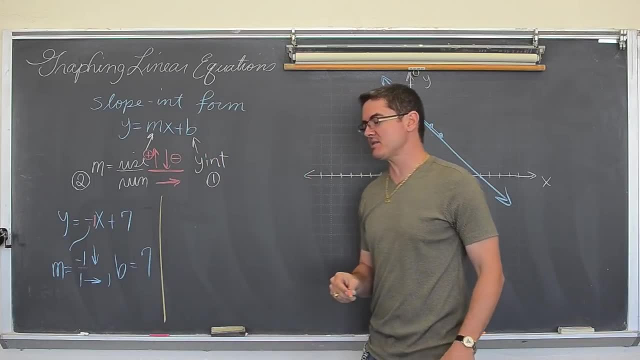 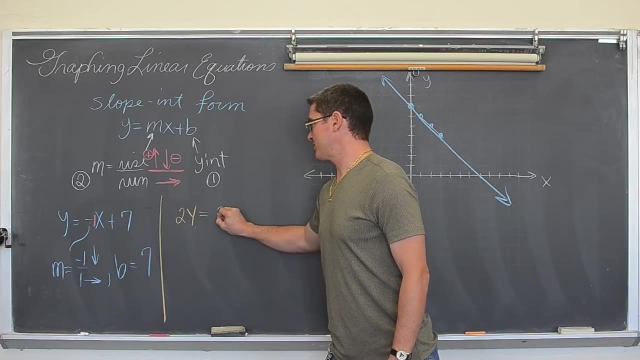 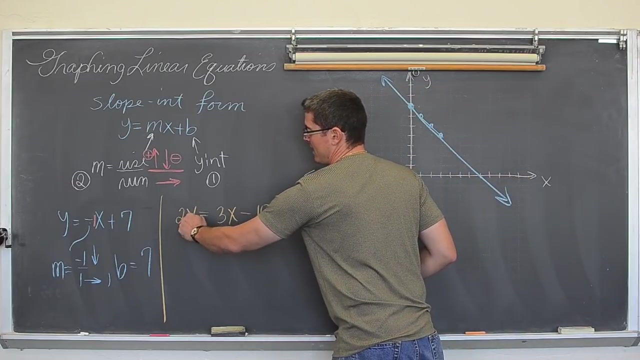 is my line. Good. Now what if the equation did not already have y by itself? Maybe it was 2y is equal to, let's say, 3x minus 10.. Well, this is close to having the y by itself, value by itself, but there is still a 2 there, So it is not completely isolated. So what? 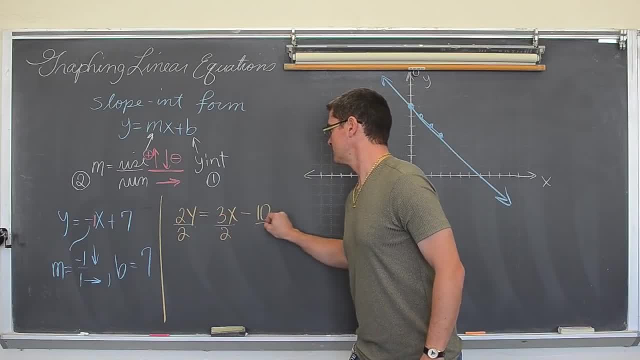 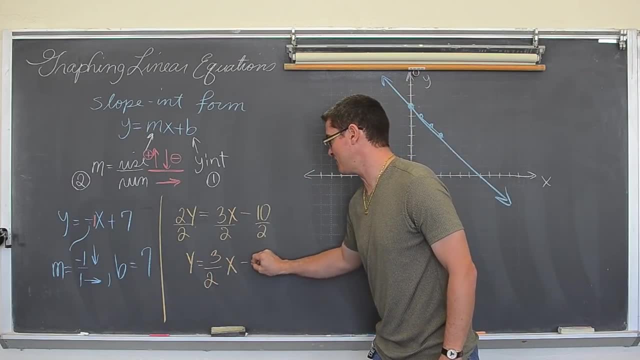 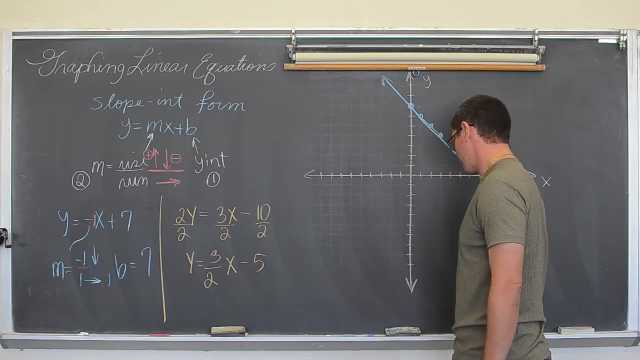 you want to do is divide everything by 2 and get: y is equal to 3 over 2x, Negative 10 divided by 2 is negative 5.. Now, because I am running out of space, I am going to erase all this in a minute, as I do the rest of my examples. My slope is in front of the x, Always in front. 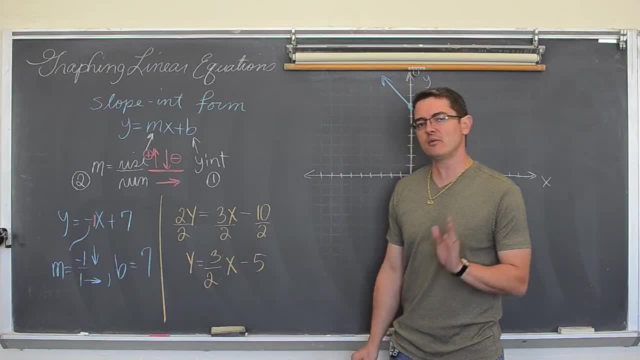 of the x. The slope is 3 over 2,, not 3 over 2x. So the slope is saying it is positive. See, there is nothing out there. so it is just a big old plus sign that we don't have to. 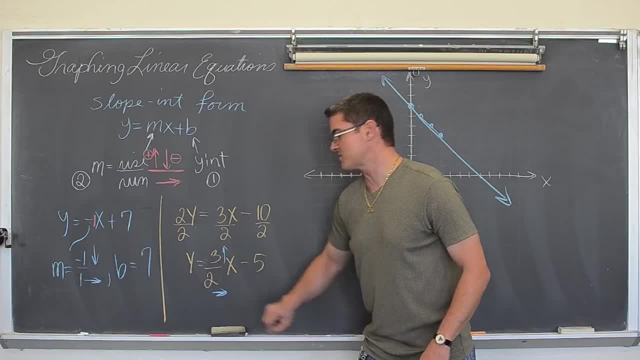 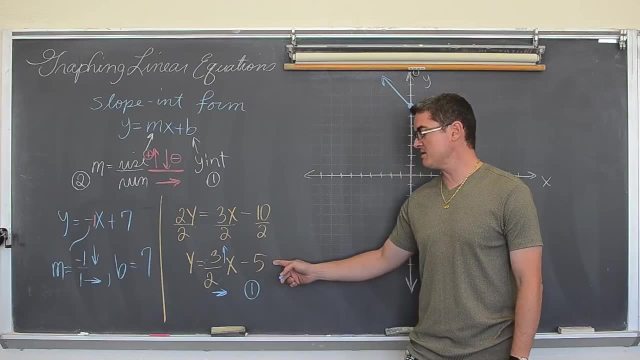 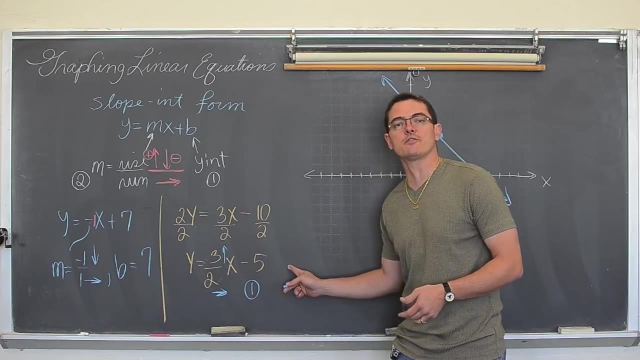 write That means we are going to go up 3 and over 2.. The y intercept of negative 5 is what we are going to do first. Again, always the last number of the constant is your y intercept. Always the number in front of x is slope. You want to do the y intercept first. 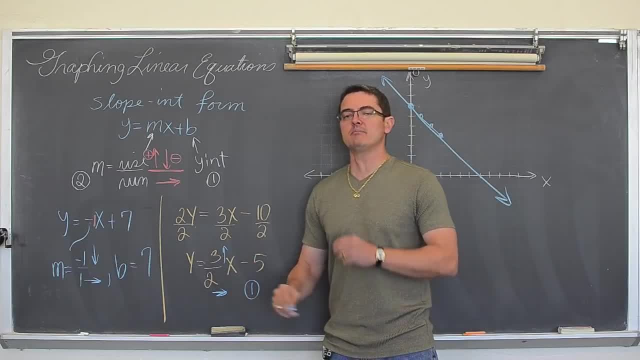 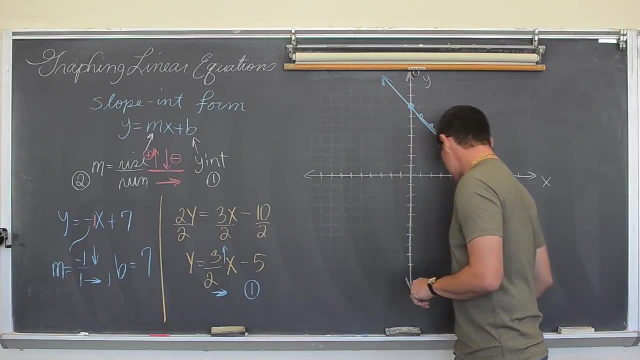 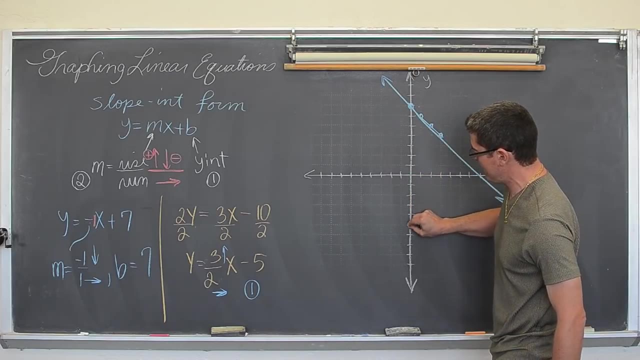 and then the slope. You can. You cannot graph a line by just visually looking at the equation, unless the y value is already by itself. One more time. So this is crossing at the y value of negative 5.. So 1,, 2,, 3,, 4, 5.. It does have a slope that is positive: 3 over 2.. So from this point, 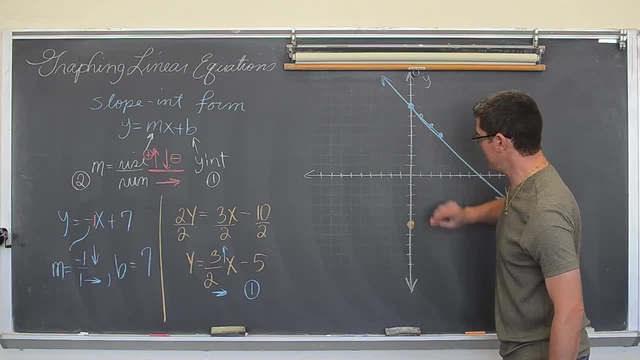 not the origin, but from the y intercept. we are going to go up 3 and over 2 and make a new point. Voila, We have a line. If you were to do a system of equations, that solution to the system. 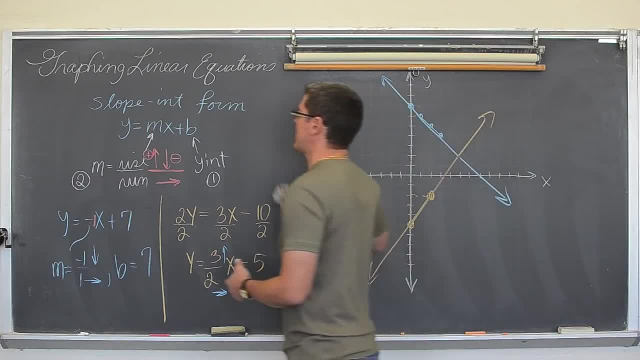 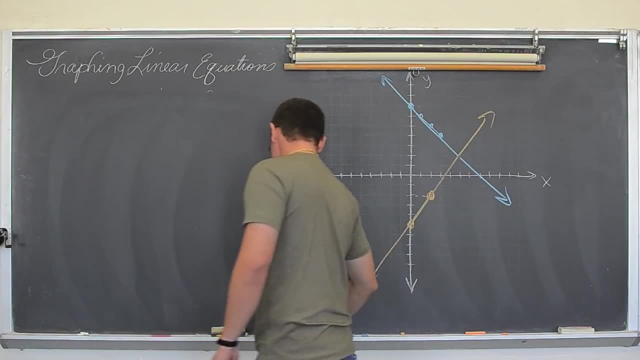 of equations would be where those two lines cross. We are not, but I am just trying to throw that out for you. Ok, one more example of a line where the equation has both an x and y value. How about negative 3y? 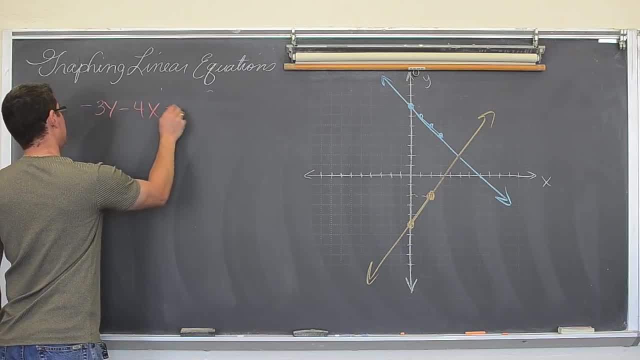 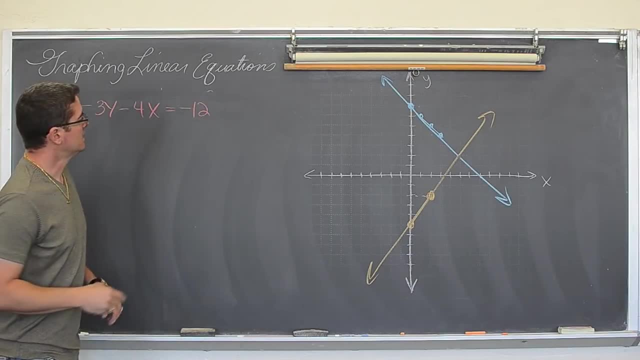 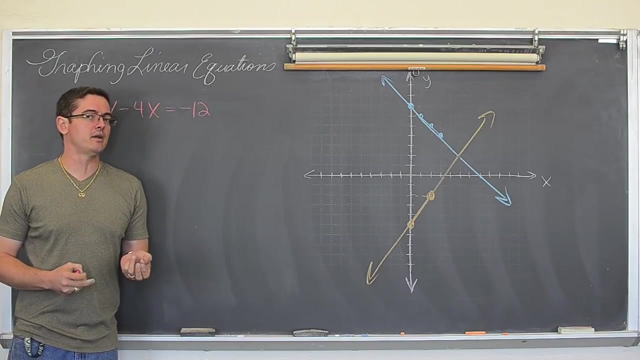 3y minus 4x equals negative 12. Everything is negative, So this is not going to be graphable, at least not without some scratch work. the way this sits, This equation is almost in standard form, and it would be good to graph this using x and y intercepts, which is what 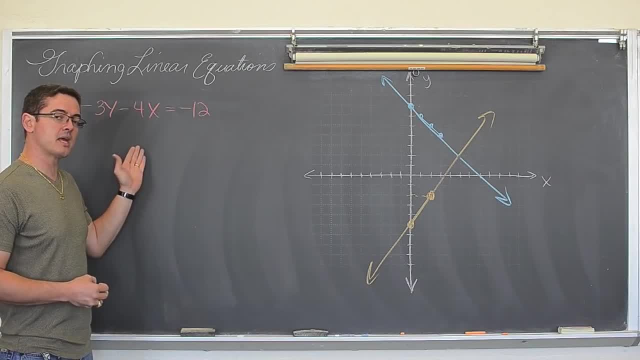 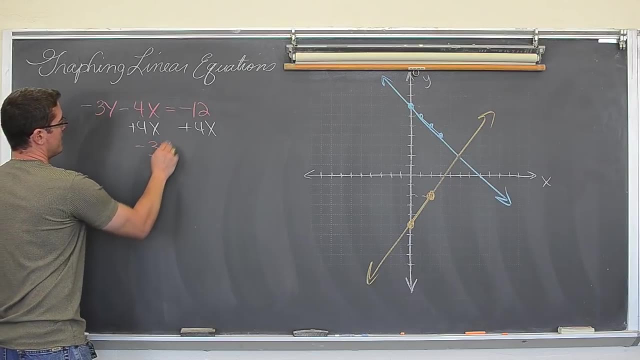 I am going to do in a minute. I want to remind you again or do another example of slope intercept form, which means the y value has to be by itself. So I am going to bring the 4x over with addition and get negative. 3y equals 4x minus 12.. Now for you algebra students. algebra. 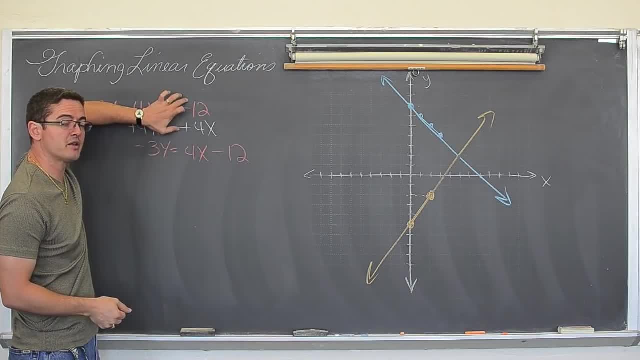 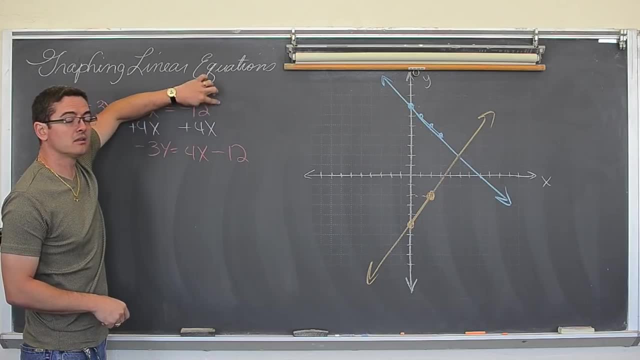 one. students remember, or please note, that I am not doing negative 12 plus 4 and getting negative 8.. That is because I am using the same equation. I am using the same equation because this does not have an x and this one does. These are not like terms, So I can. 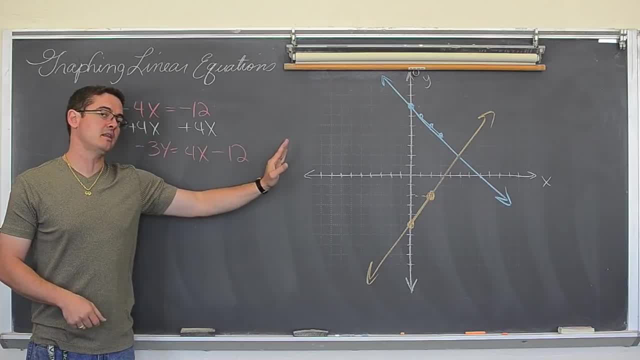 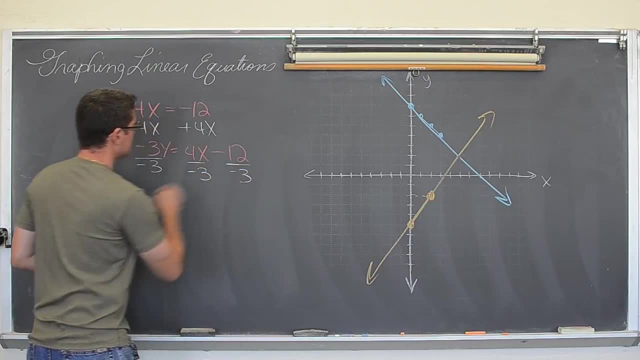 just show those two terms together on the right hand side of the equation I cannot actually put them together. Dividing everything by negative 3 and we get y is equal to negative 4 thirds x plus 4.. Now you may note that this negative here when I divide everything by. 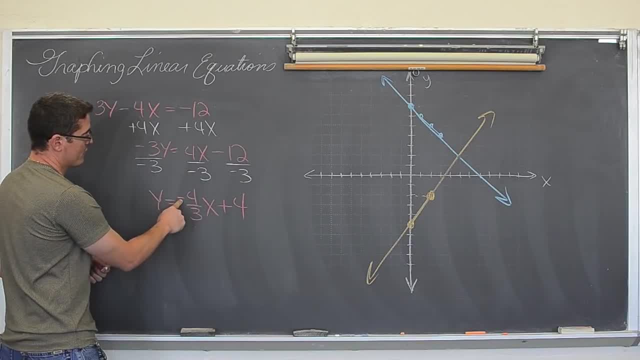 negative 3, the negative is on the bottom of the fraction. What I am going to do is I am going to divide by the negative 3.. I am going to divide by the negative 3.. This fraction Now I have written it on the top. That is because it doesn't matter where you. 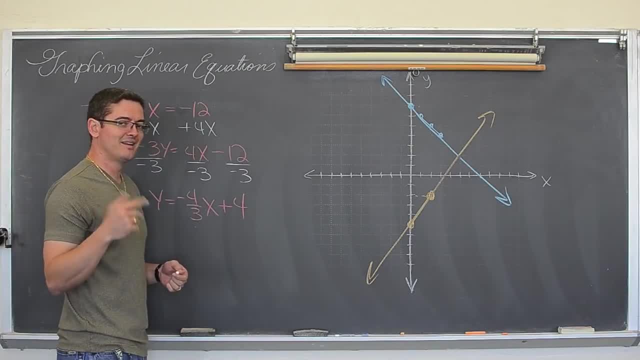 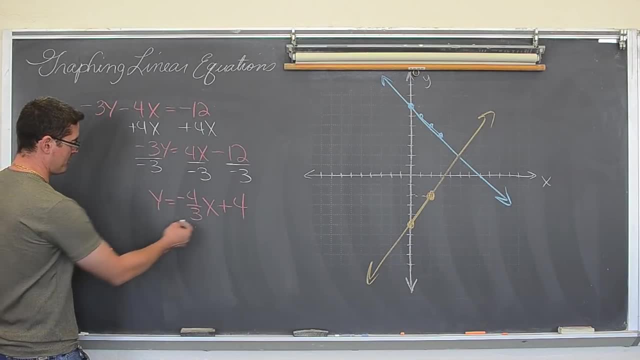 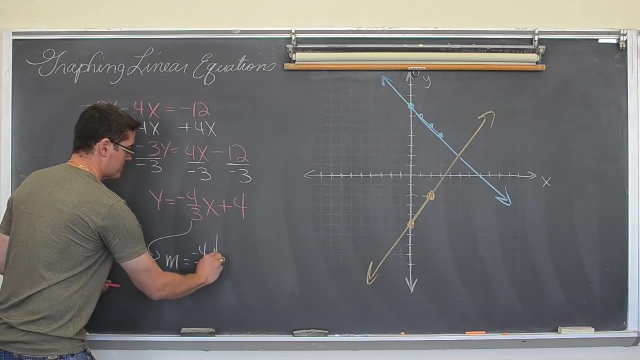 write the negative sign. You can put it anywhere you want, as long as there is only one negative sign in the fraction. Ok, so now y is by itself, So I can find the slope which is in front of the x. That slope is negative four thirds, So we are going to go down four and over three. 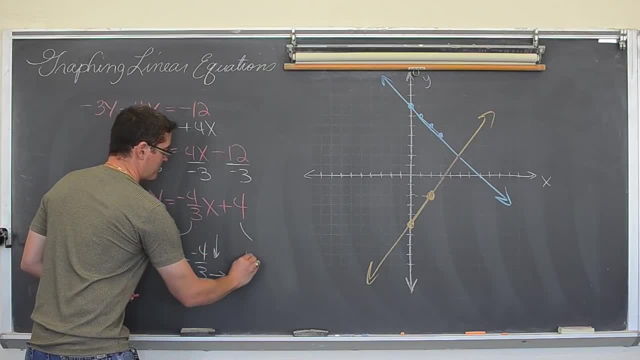 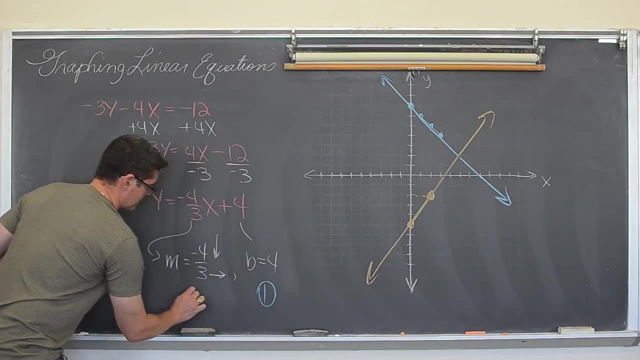 And the y intercept always is the constant at the end of the question. So b the y intercept is equal to four, And again you want to do the y intercept first and the slope second. This is going to be a busy graph over here, so I will be erasing it in a minute, But I 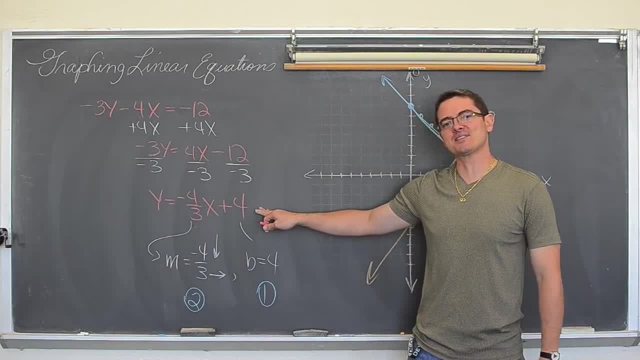 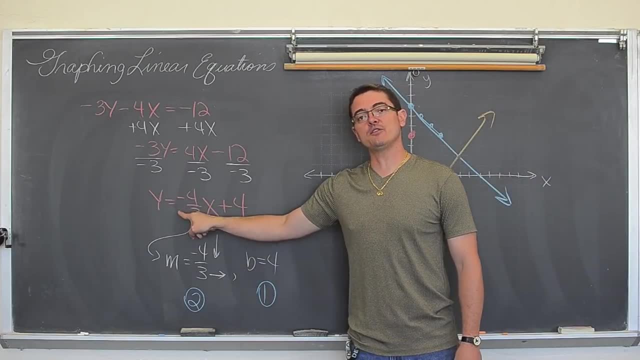 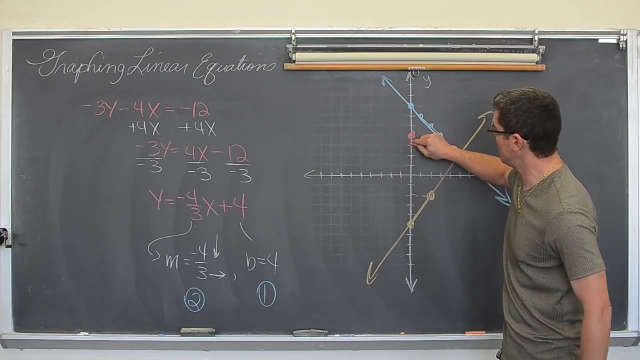 think I can put one more on here. This line crosses the y axis at four. So one, two, three, four. This line has a slope of negative four thirds. So again, the rise over the y axis and the run means down, and the bottom should always be to the right. So down four. One. 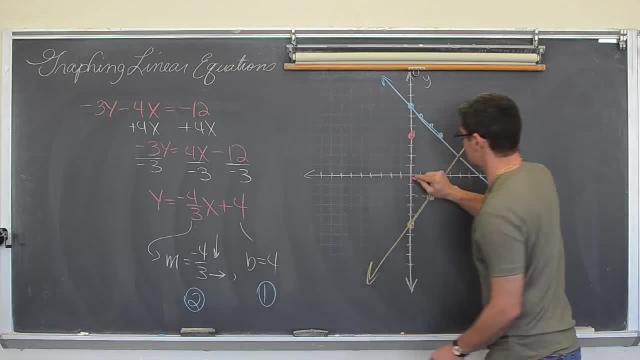 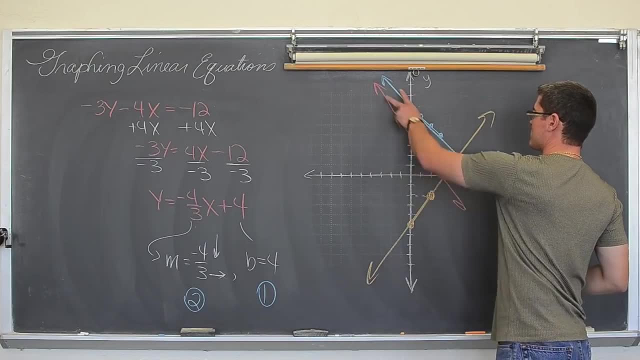 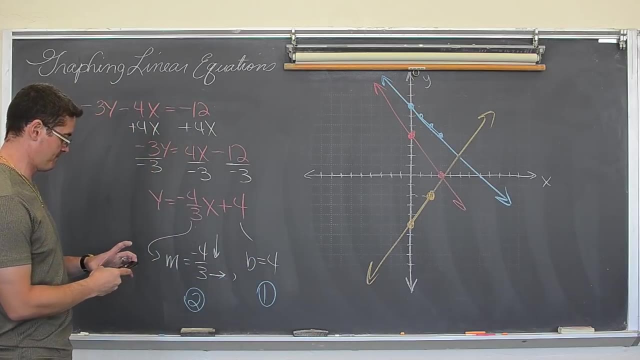 two, three, four And over three. So one, two, three, And we have this line. It looks like those are almost the same slope, but they are not. So that is three examples of how you graph lines in slope intercept form. Ah, I have a few minutes left. Ok, let's talk. 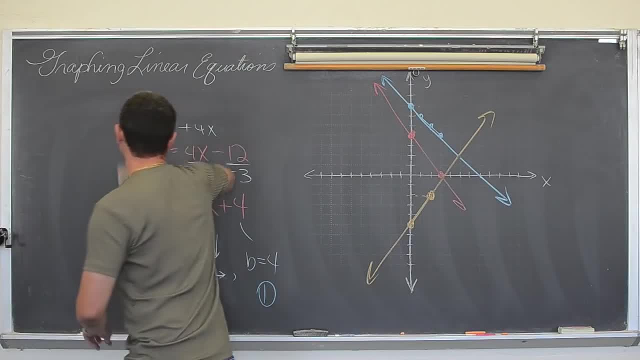 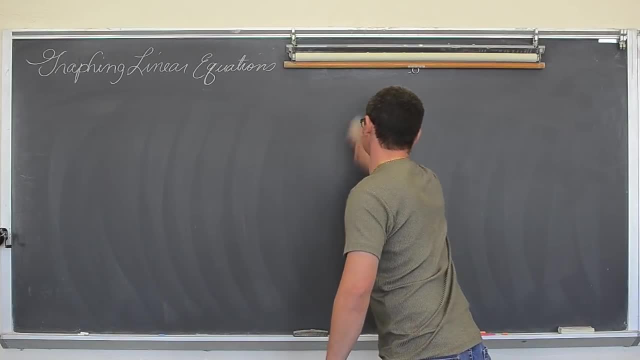 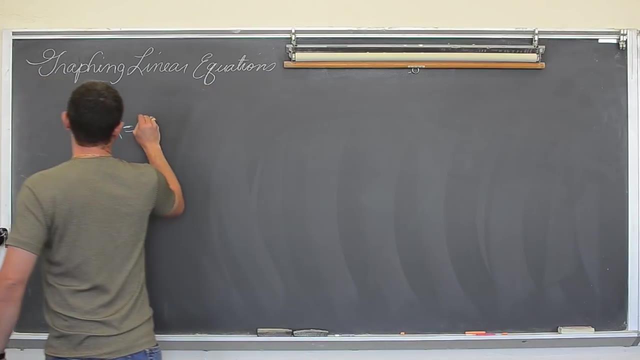 about? what is it? what do you do? how do you graph lines in slope intercept form? How do you graph a line when you don't have both an x and a y value Like, how do you graph the equation x equals four? It is like there is not even enough there to do These questions. 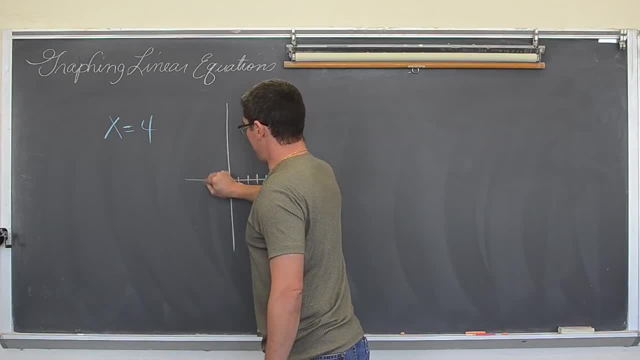 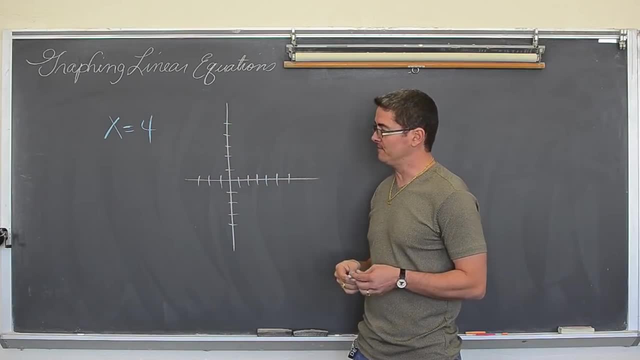 as math teachers, we kind of hope are the easy ones, but because there is so little going on in the equation, it is almost like there is nothing going on. It is almost like there are mistakes actually more often. x equals four. There is not x and y. We are not sure. 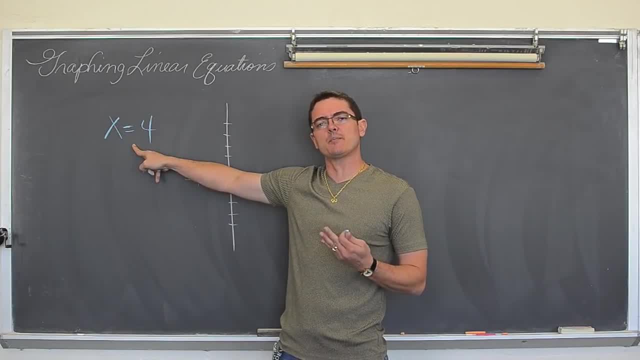 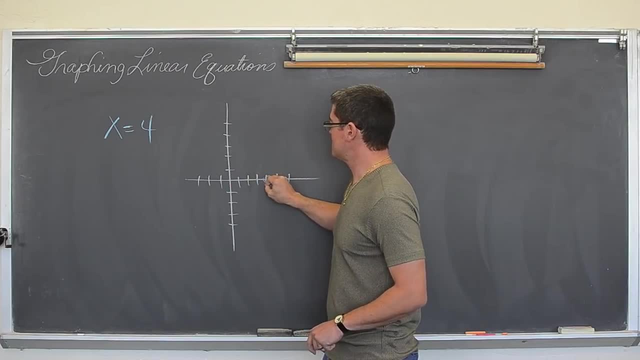 what this is like. Well, if you are graphing lines, just think up a couple of points with an x 😈 of four, like four zero. Alright, So some losing ones. Four zero, That has an x 😈 of four. Think up another point that has an x: Liberally two. Four two That has 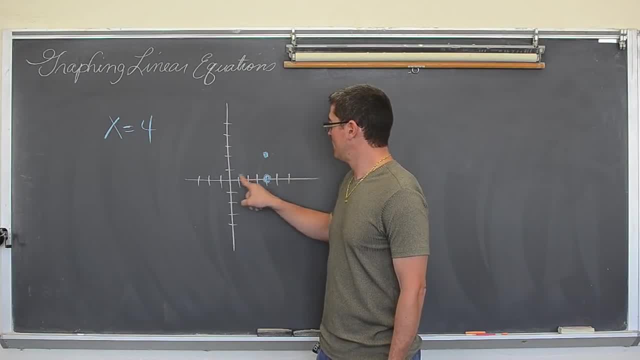 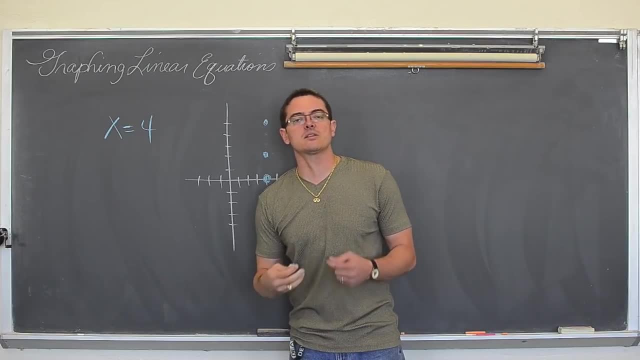 x coordinate of 4.. How about 4, 5? 4, 2, 3, 4, 5.. Well see, what I am doing is: I am coming up with points that all have a coordinate, an x coordinate of 4.. Maybe I forgot that?